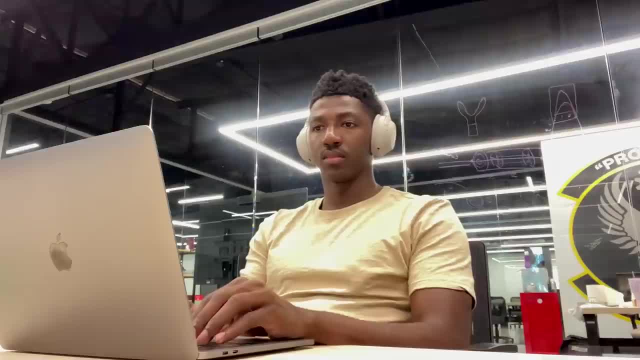 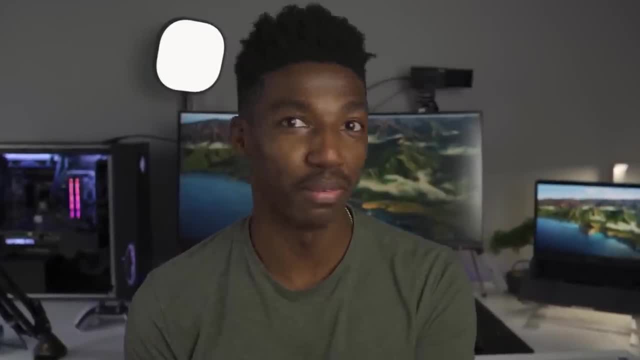 Yo, welcome back to the channel. My name is Jeremiah Peoples and I've been doing this software engineering thing for about three years now, And before I got started, there's a ton of things that I wish I would have known before hopping and trying to dive into this career field. 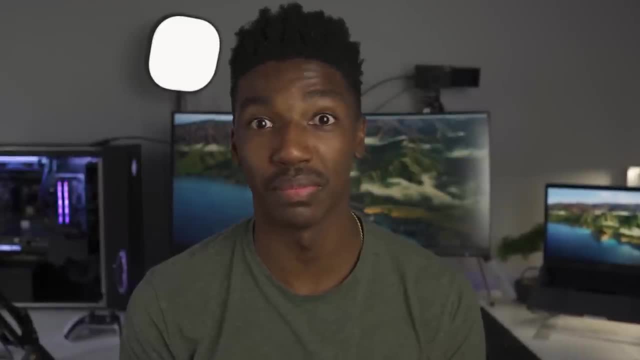 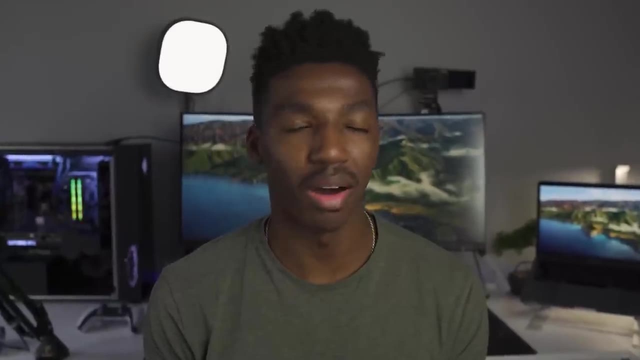 So this video is all of the things that I wish I would have known before starting to dive into software engineering. condensed into one video that is in a rectangular shape. I had no idea all the different ways a person could learn how to code, So, obviously, going to a four-year- 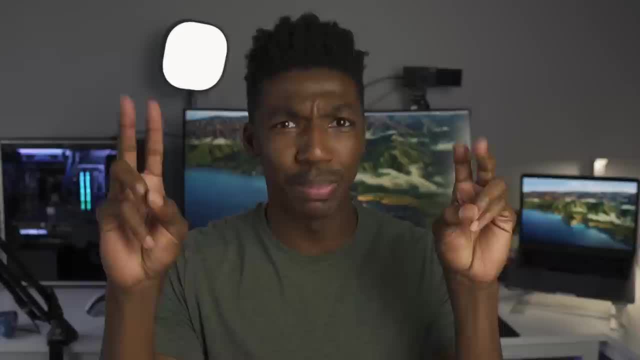 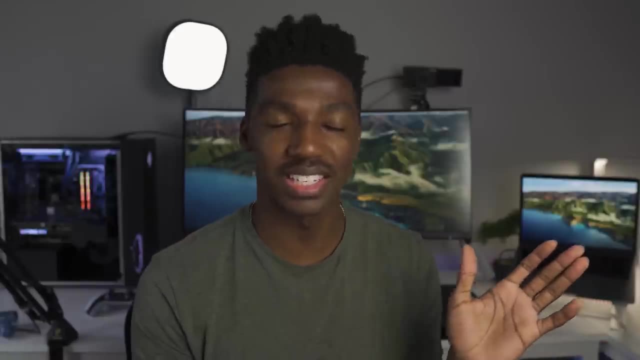 institution and studying computer science is one of the most typical ways to become a software developer or software engineer. For me, that's what I try to do. I try to go to college and learn computer science stuff, but I dropped out because that environment wasn't really for me and it 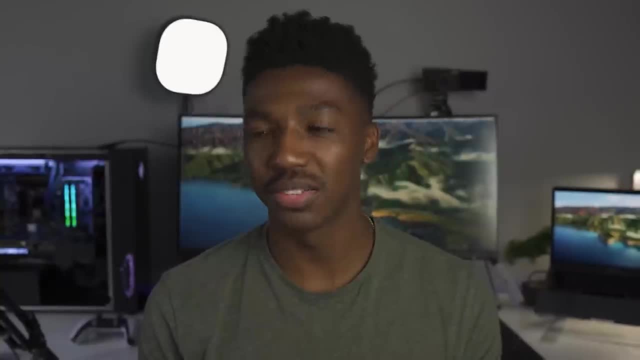 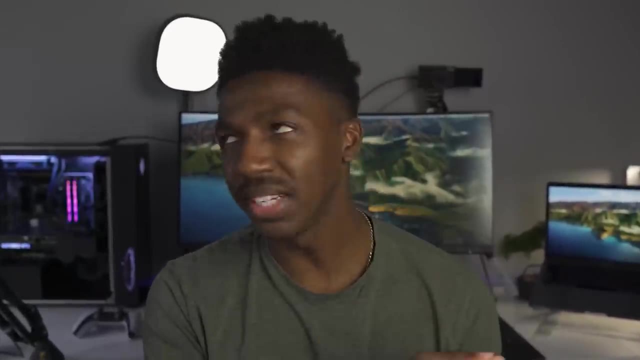 wasn't really how I liked learning how to code. So when going to college for computer science didn't really work out for me, I thought, oh well, that's it, I guess I'm not going to be a software engineer. And then, three or four years after I dropped out, I was pleasantly surprised. 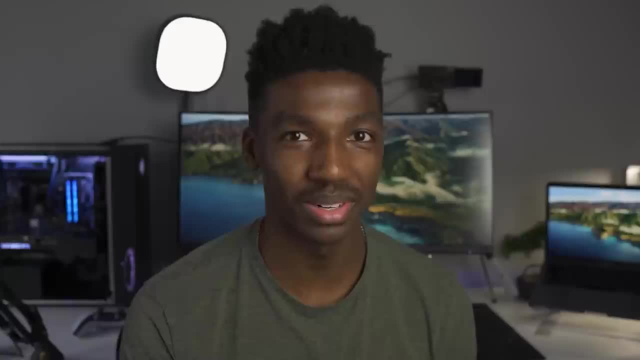 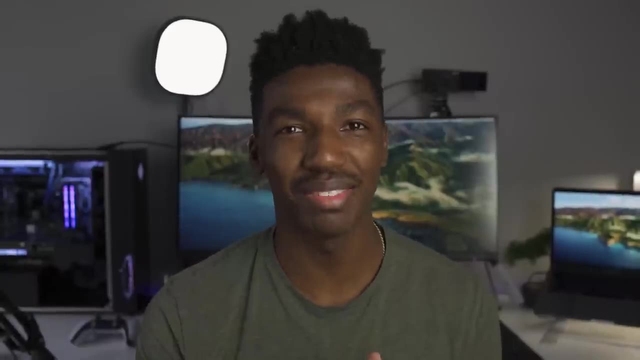 to figure out that you don't necessarily have to go to a four-year university study computer science to be a software engineer. Who would have thought So? three or four years after I dropped out of school for my computer science degree, I stumbled upon a video of this guy named Chris. 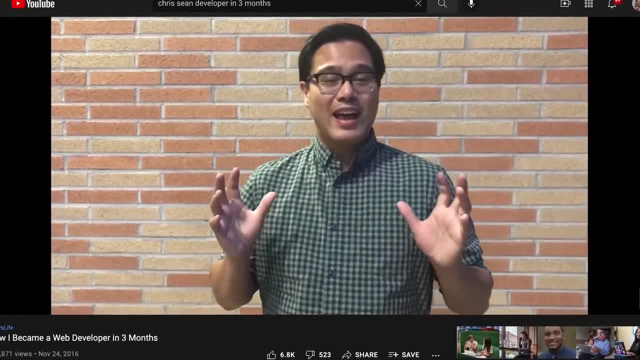 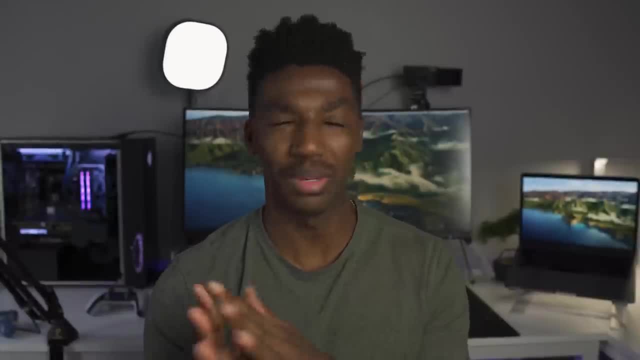 Sean, who is now my friend, about how he became a software developer in three months without a college degree, And I was intrigued, to say the least. So in that video that Chris Sean posted three or four years ago, he talked about how he was a self-taught software engineer, And I was. 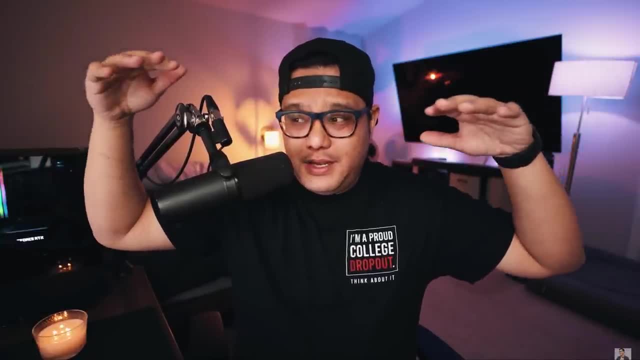 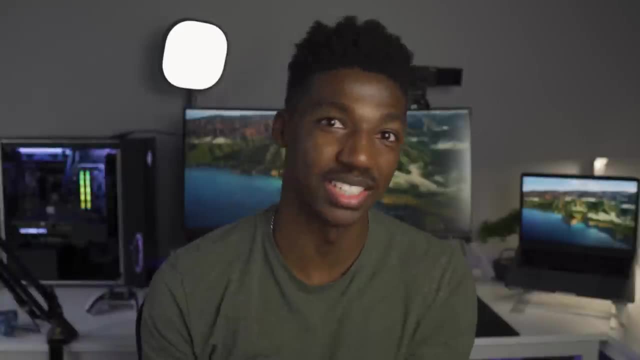 like, wow, he's a self-taught software developer. He didn't go to college And that was that was um. that was interesting to me because he was doing the job I wanted to do And he circumvented the going to college thing, which was pretty impressive. So I am incredibly fortunate. I. 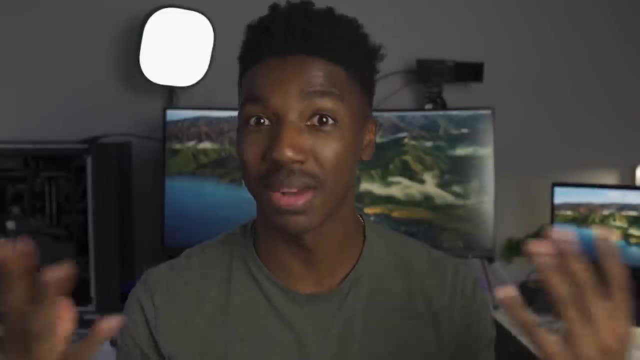 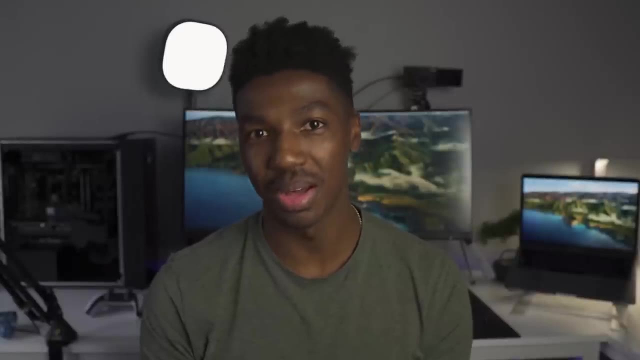 stumbled upon that video, or the YouTube algorithm pushed it in front of my face, because I am now currently a self-taught software developer, just like my friend Chris. So, moral of the story, what I wish I would have known on my first day of programming was all the different types of 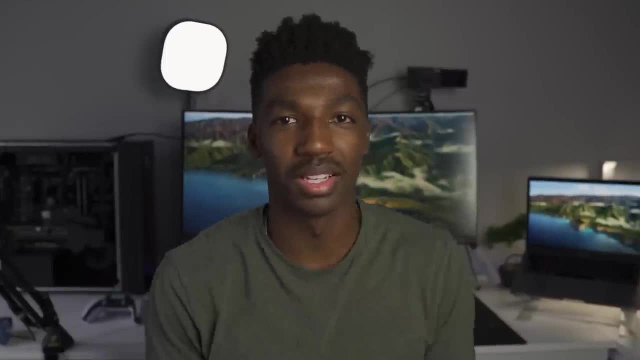 pathways that you can do to become a software engineer, And that's what I'm going to talk about today. So what I'm going to talk about today is how to get into the software development career field. So obviously I talked about the basic one, which is getting your four-year bachelor's degree in 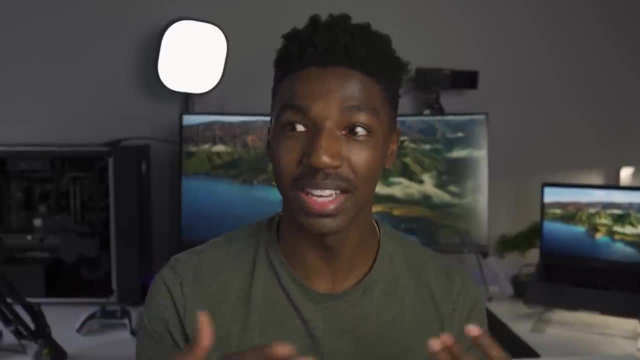 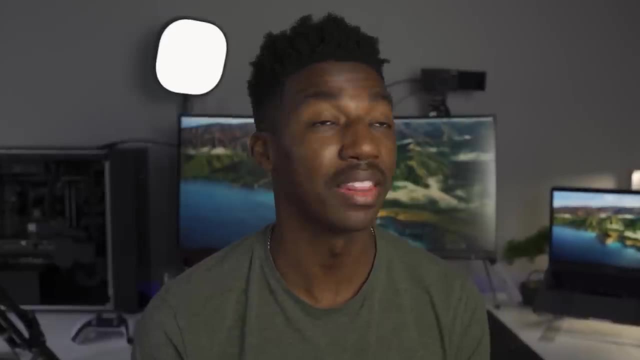 computer science. And then there's the self-teaching way, which me and Chris did to, where you just go online and look up all the things that you need to learn to become a software developer. And there's the coding bootcamp, Like I mentioned earlier, coding dojo. you can go to a program for three. 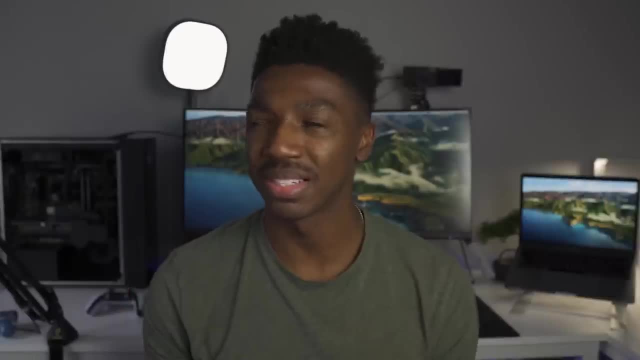 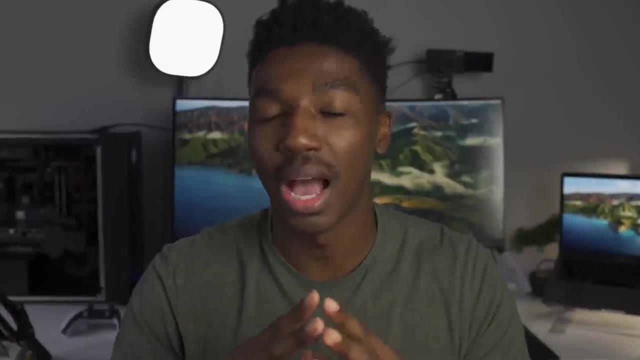 or four months and learn to code from them. But when I first heard about self-teaching and coding bootcamps, I was like there's no way you're at the same level of these people with degrees. I was pleasantly wrong about that In my almost three years of experience as a 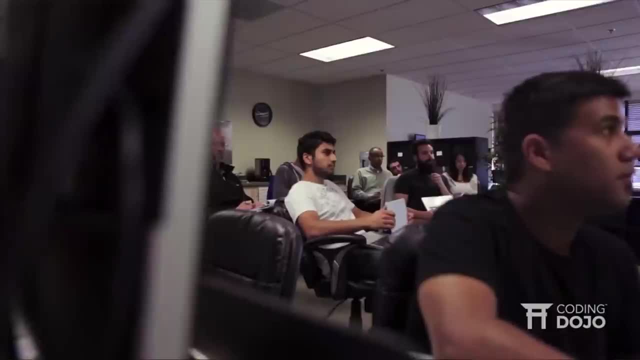 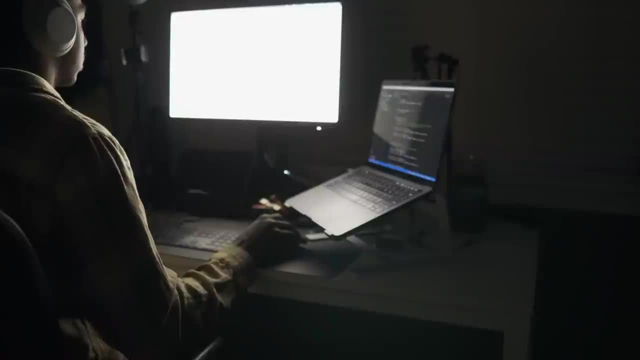 software developer. I've worked with a ton of different people, some from coding bootcamps, some from degree programs from prestigious colleges, and some that were self-taught like your boy, So that's another fun thing that I wish I would have known was. 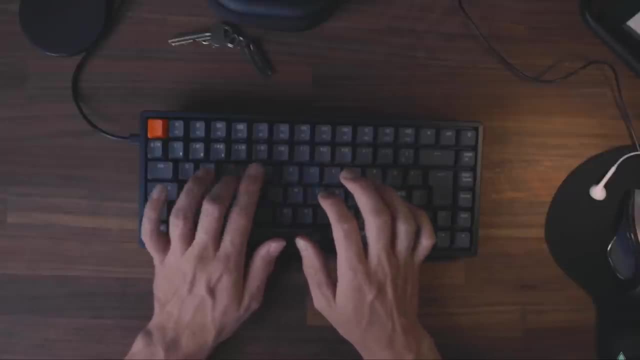 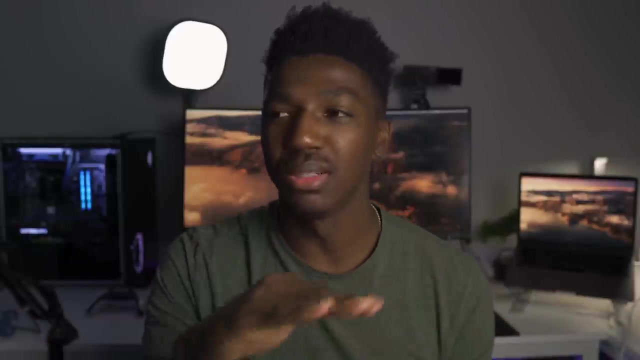 hey, it doesn't matter where you went to college or where you learned to code. You're going to be treated as an equal to every one of your peers And, speaking of getting paid, the absolute same for doing the same job, regardless of your 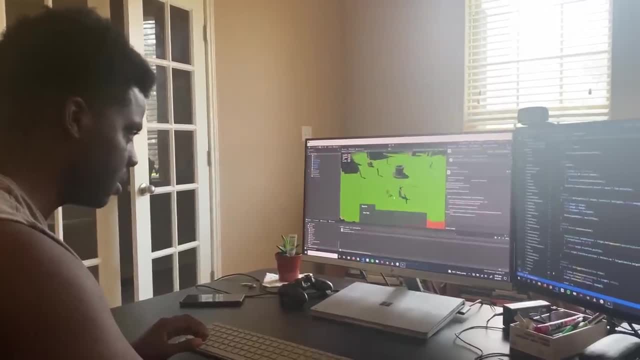 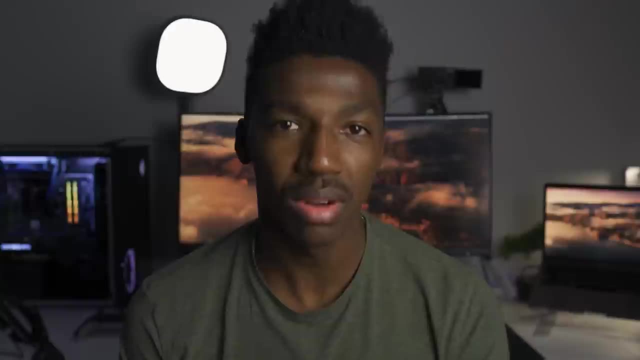 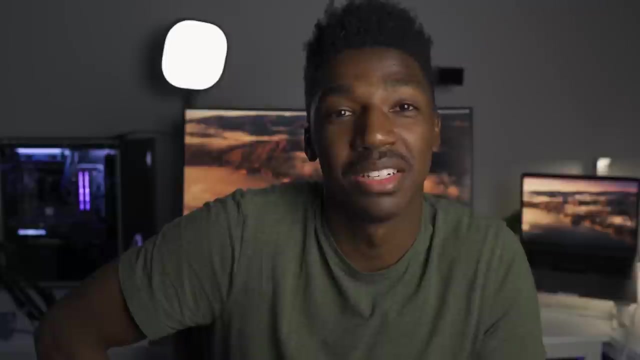 background asterisk: I am very upset that my brother, who is also in tech, was keeping the pay a secret. So this brings me to my next. what I wish I would have known before starting programming that the pay goes absolutely stupid, straight, dummy, straight, thick. They'd be paying money. 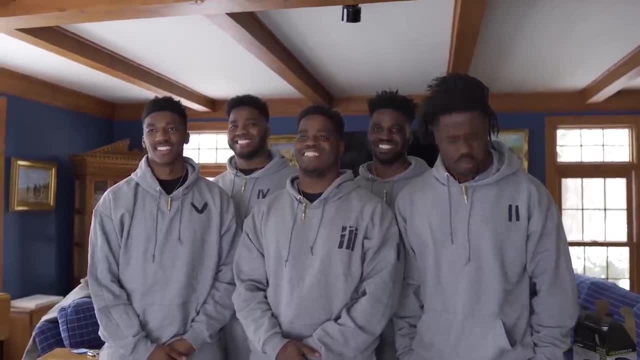 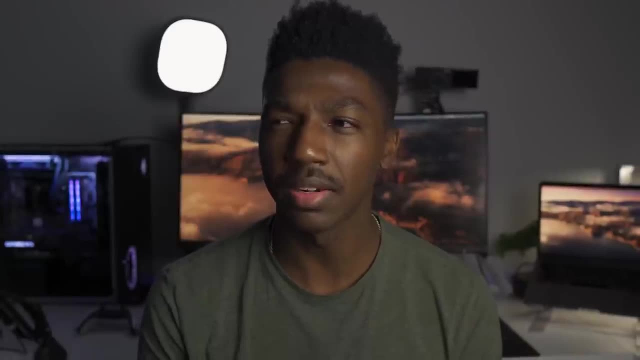 to do this coding thing. My brothers don't Know it, but I'm in a unconscious race with them to become a millionaire before any of them become millionaires. But I feel like they're not telling me tips and tricks about life. They're. 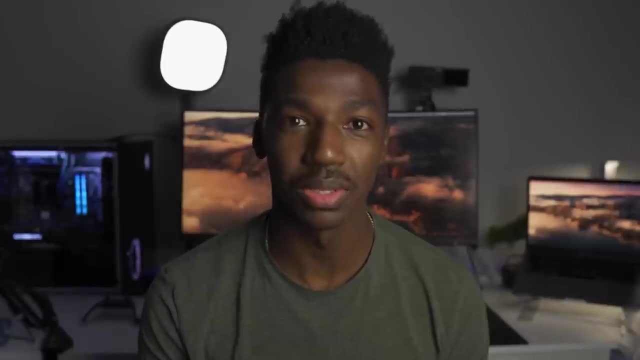 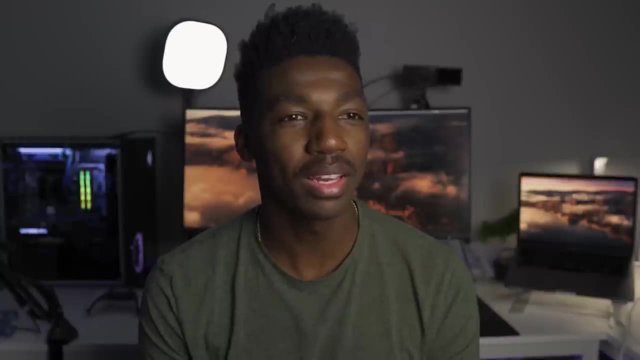 all my older brothers. So I feel like my eldest brother, Josiah, who's also in tech, not telling me that the pay and software development goes stupid. Um, he's trying to. he's trying to get a headstart on me, which is not fair. I don't respect it. Josiah, I'm coming for your head. 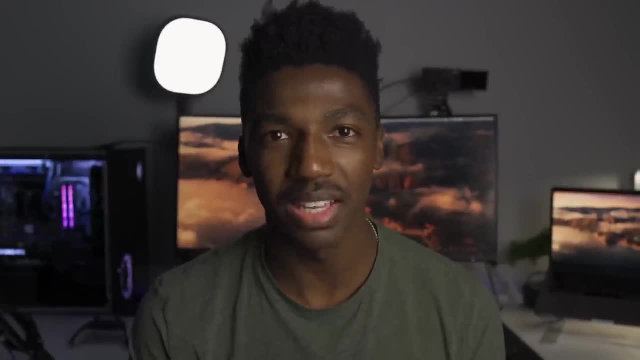 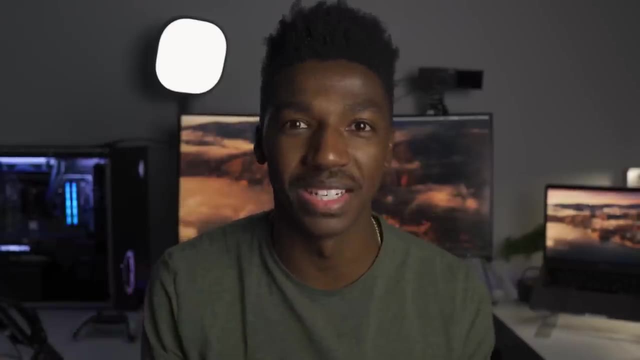 You know how, when some people are just sitting on the couch board, as can be- they hop on Zillow and they just look at houses that they can't afford. but they just like to house shop for no reason, because it feels good. I started doing the same thing on this really cool site called. 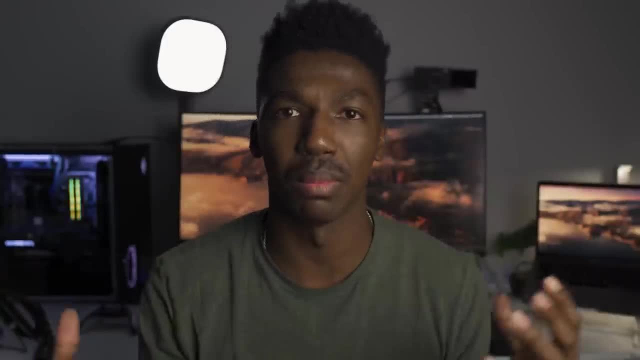 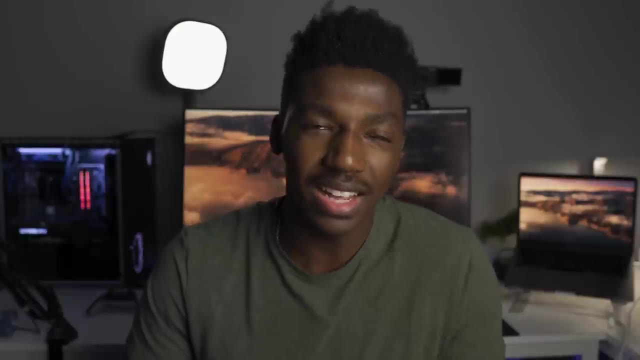 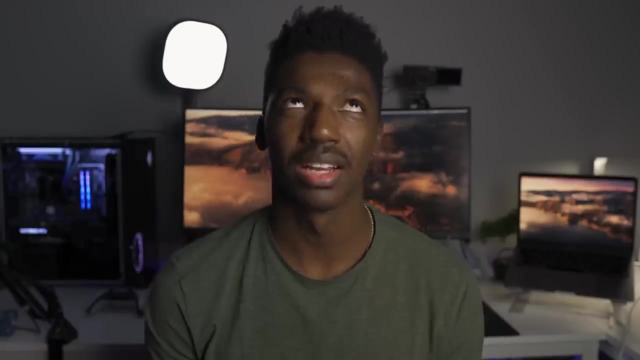 levelsfyi. It has a bunch of different like reported income salaries. So, for example, I would hop on to levelsfyi and look at, look at, look look at this for Slack, to start off as an entry level software developer, at Slack It's 176. hop over to DoorDash, entry level is 196.. 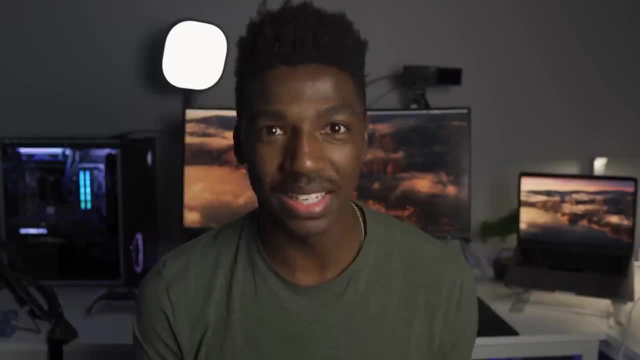 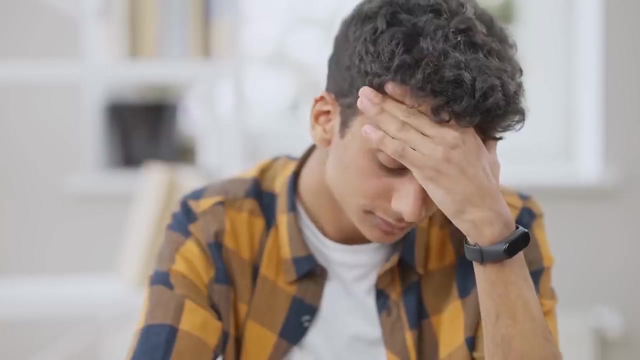 Look, entry level, It's like 185.. It's ridiculous And it was so weird to see that people were paying this munch munch this much for people who know how to code. Whenever I was struggling learning a new concept, I was going through it, I was like: is this really worth all this headache? 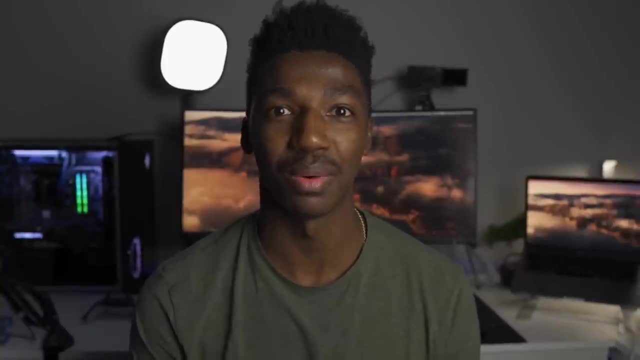 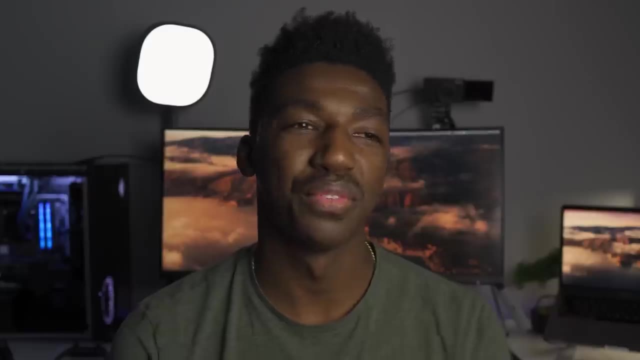 that I'm having to go through. I would hop my happy little butt on levelsfyi, scroll through a couple of the job payments And I'm like, yep, this is definitely worth the headache. So very rarely, though, if you're starting to hop into this career field, you're going to hear these. 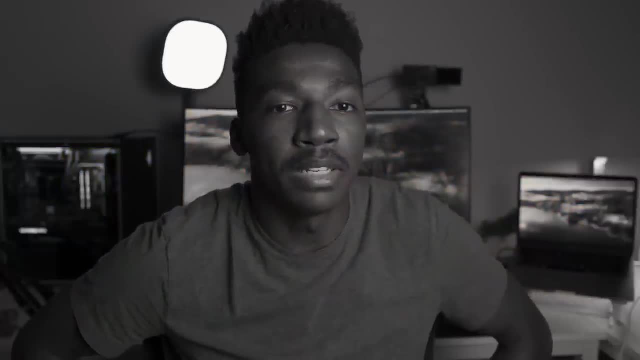 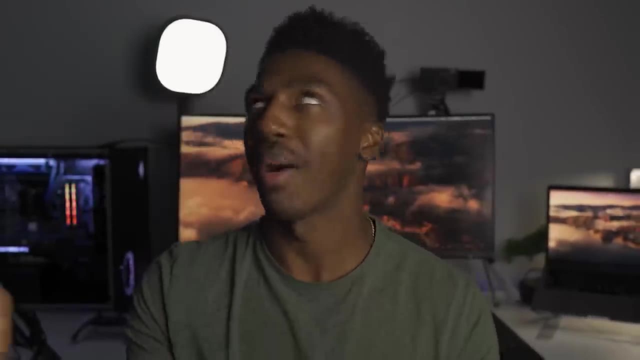 internet trolls say: well, you shouldn't have me doing this for the money. Back in my day, I did it for the love of binary. Just realize that those people that are grumpy and frumpy, that you don't love binary and pointers and that's your only driving factor to become a 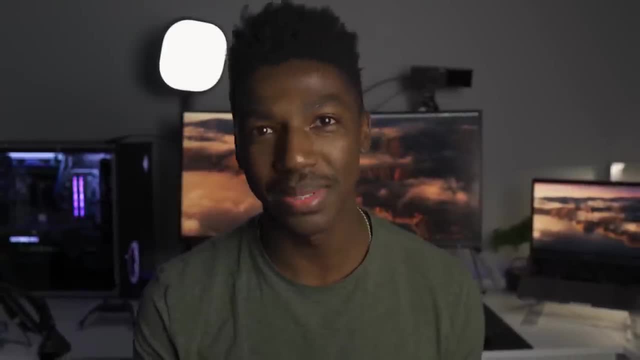 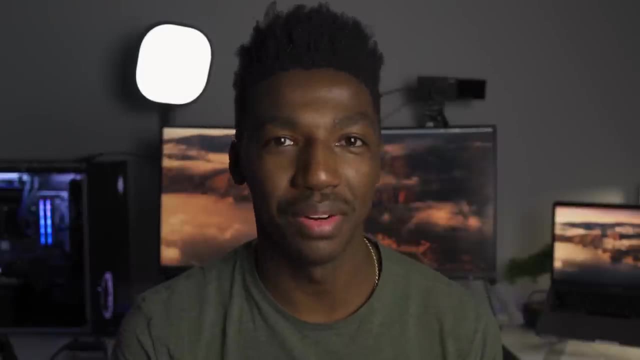 developer. Those people are trolls. They're not very common in the developer community. I don't think I've met any in person. There is absolutely nothing wrong for wanting to hop into this career field because it has a very promising and exciting salary. It's so weird that people are online. 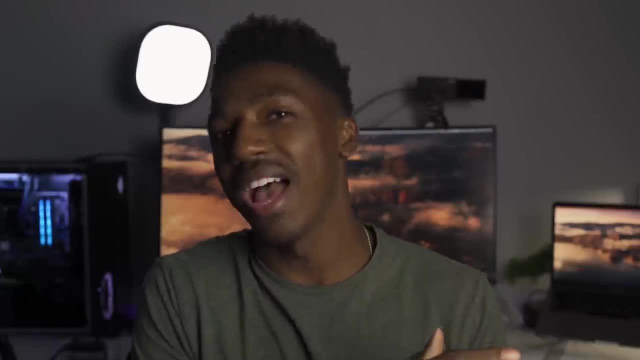 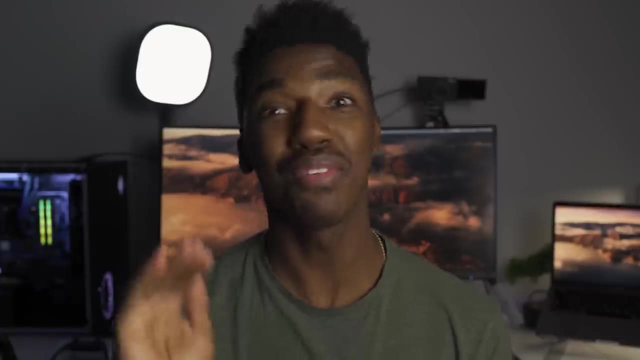 saying, well, you shouldn't be doing it for the money when the money has the chance to change your life, change your whole, entire path of your life and your family's life. So to look over that fact and to just be like, well, I'd actually love ones and zeros and that's it. That's kind of silly. 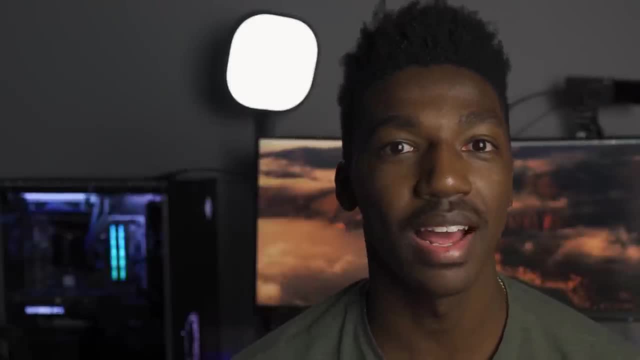 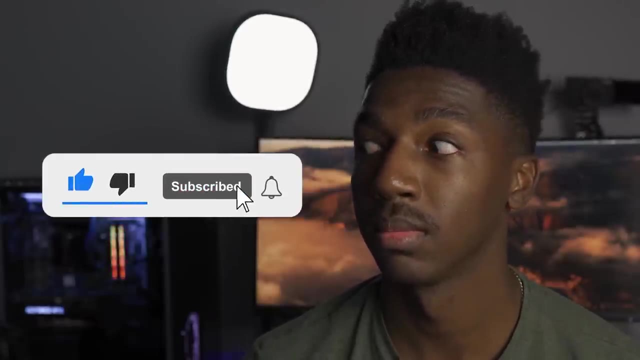 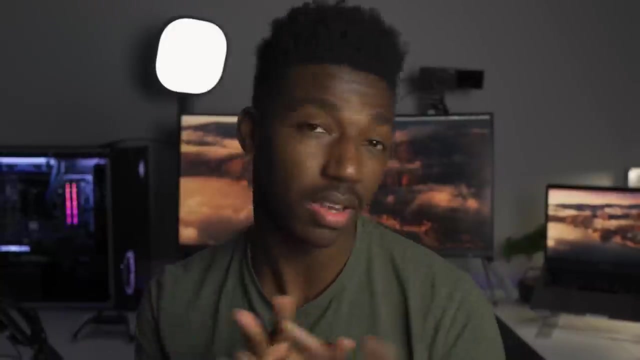 So what I didn't realize until very recently is that the internet has a lot of nice folks on it And if you ask them to like your video and subscribe if they enjoy your content, they actually might do that. So I know, but for real, the next up is this job, this developing code and writing software. It's 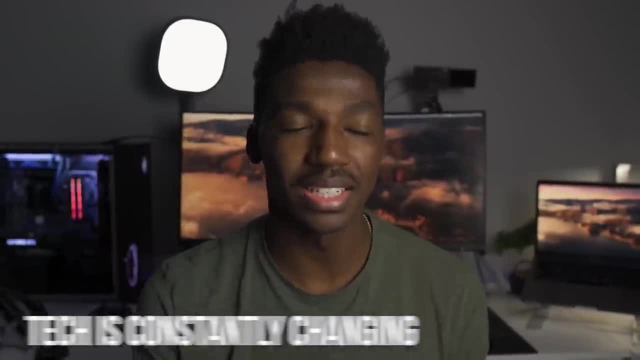 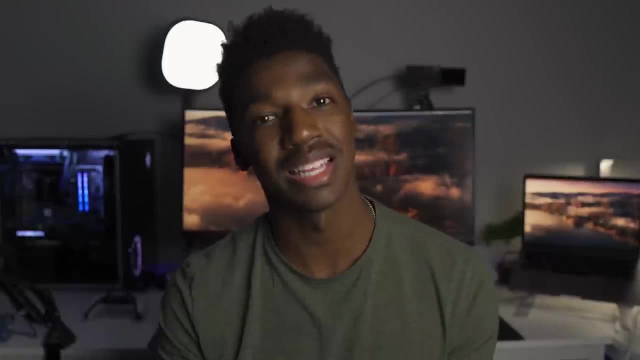 it's not easy, And software development as an industry is always constantly changing, which comes with a lot of pros and a lot of cons which I wish I would have known. So that's why it's in the video And that's why I'm going to say it to you. So if you spent more than five minutes, 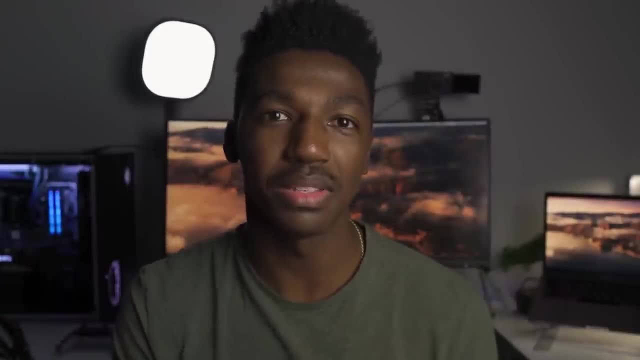 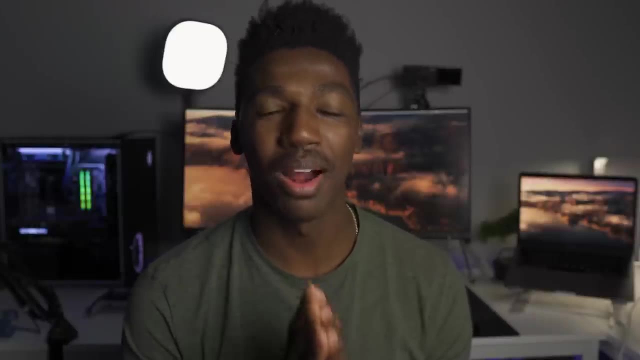 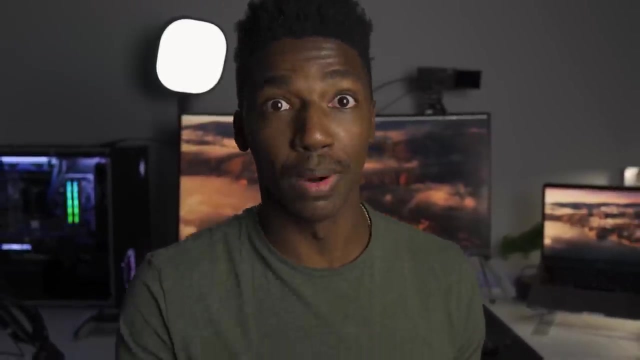 thinking about hopping into the world that is software development. you know that this career field isn't- um, what's the word? It's not easy. It requires a lot of work and a lot to wrap your mind around, And I'm not saying that in a gatekeeper way, like well, it's super hard. 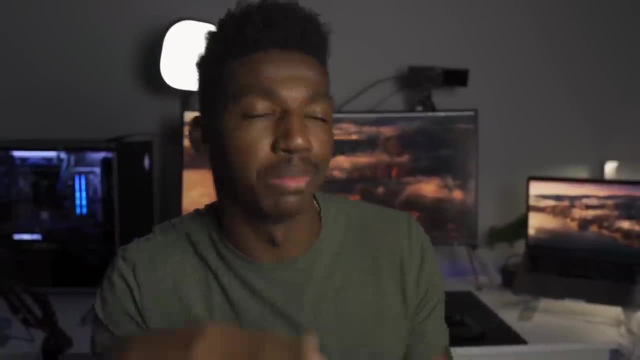 but I mean I, I do it, but it's super hard. You probably won't be able to do it, but I but I do it. I'm not saying it like that at all. I'm saying it more to prep you, because if you have the right, 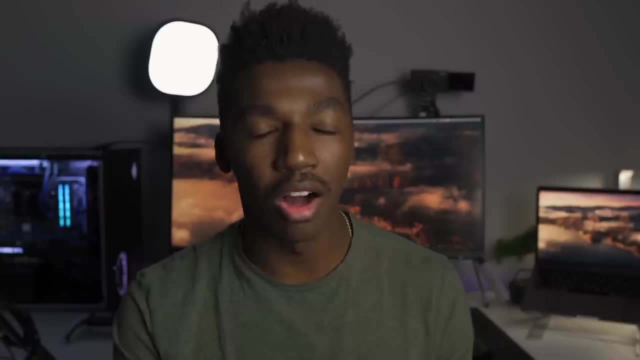 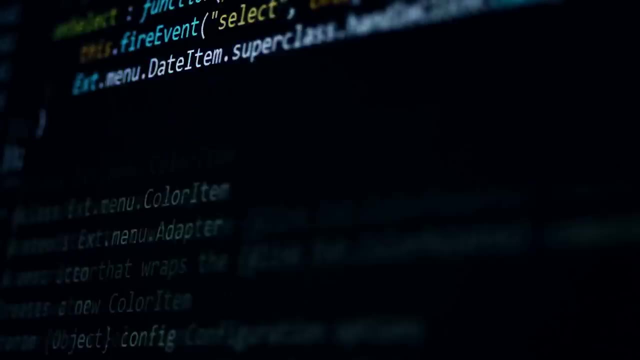 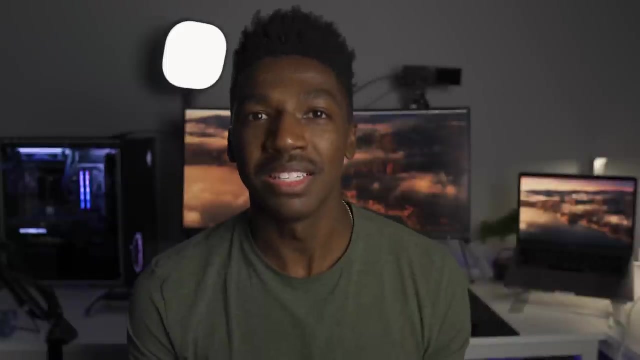 mindset before trying to get in this. you're more likely to conquer the lines of code that are mysterious to you at this point, And if you've never seen a wall of code before, it's it's going to be pretty, pretty terrifying and pretty hard to get your mind around. but nothing good comes easy. 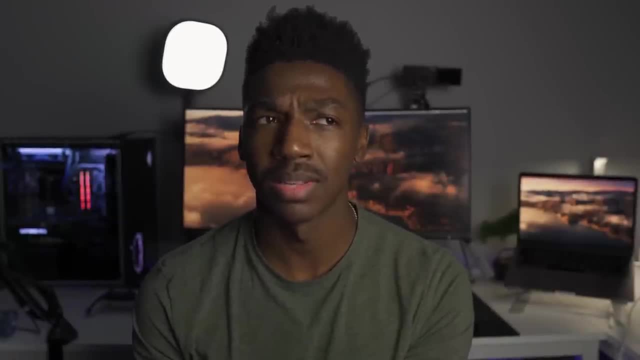 So if it's hard, that means it's great. right, That's the. that's the logic there. Okay, cool, We get it. Coding is hard. That's that's nothing new. You probably knew that before watching this. 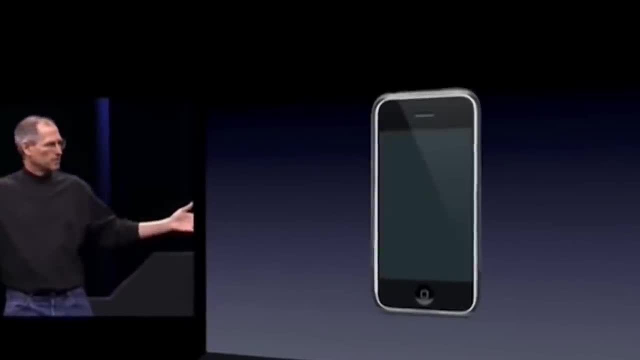 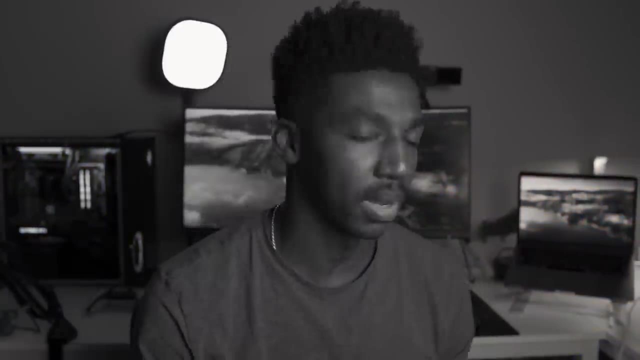 because how frequently the community, the languages, the technologies surrounding software development changes the whole world. Do I have a globe in here? No, I just have to use my hands. The whole world is constantly evolving, and it's constantly evolving because it's being driven by. 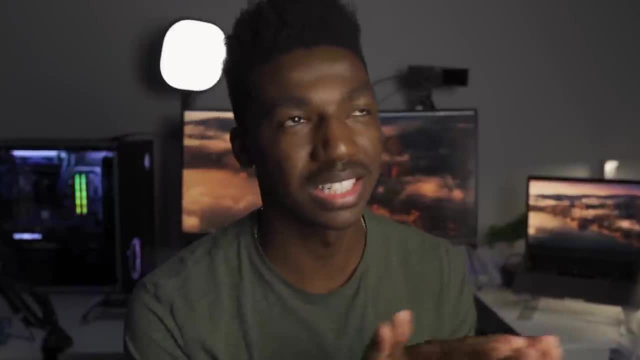 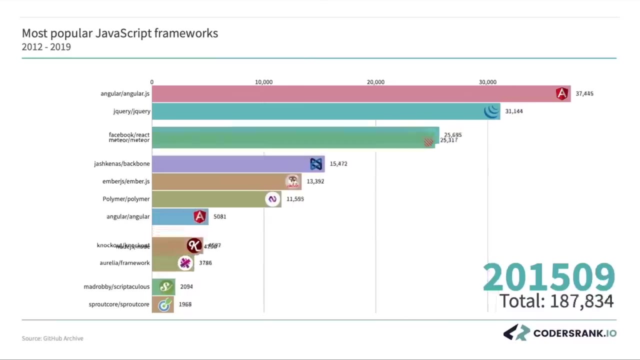 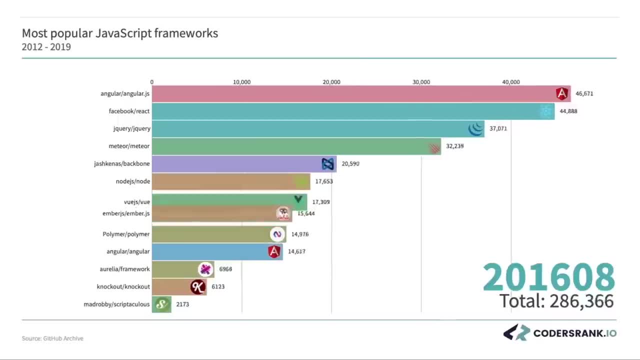 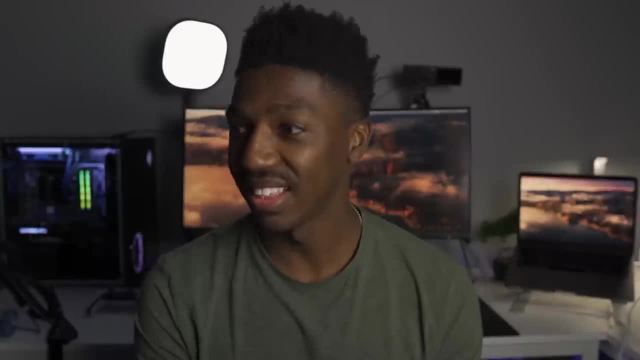 in the next six months, that language or library could be obsolete, No one ever uses it, And now you have to learn another language or library just to stay relevant. So that, right there, I was very unprepared for of how fast things can get deprecated, how fast things can fall out of. 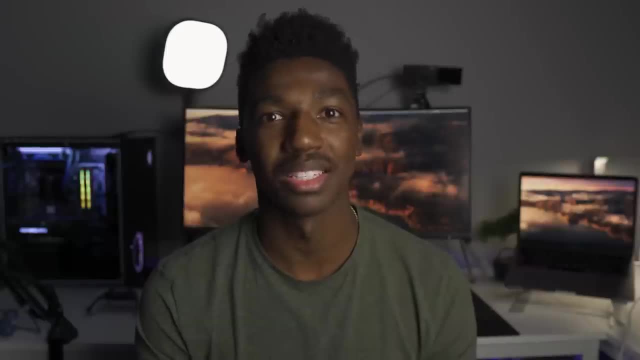 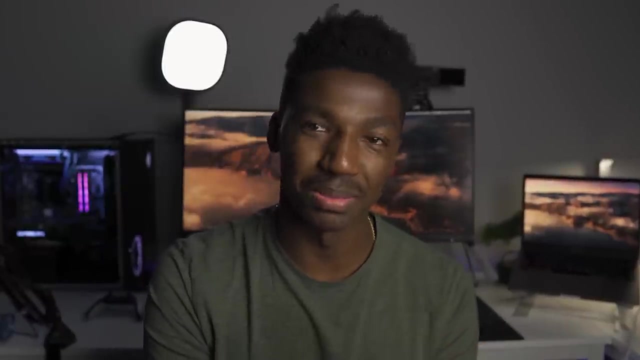 being the hot new thing. I didn't know that before hopping into this career field, but having a career field that is rapidly evolving has its pros and cons, which I'm going to share with you. So what I'm about to say next, depending how you look on it, can either be a pro or a con. 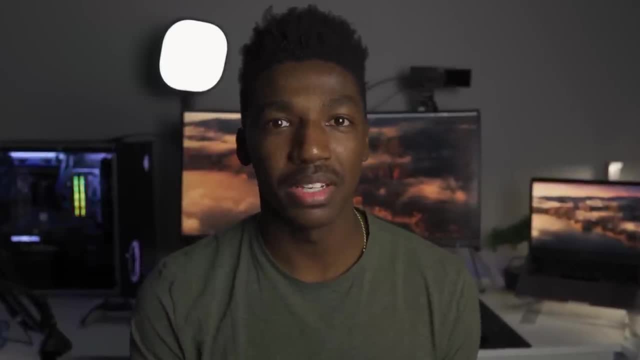 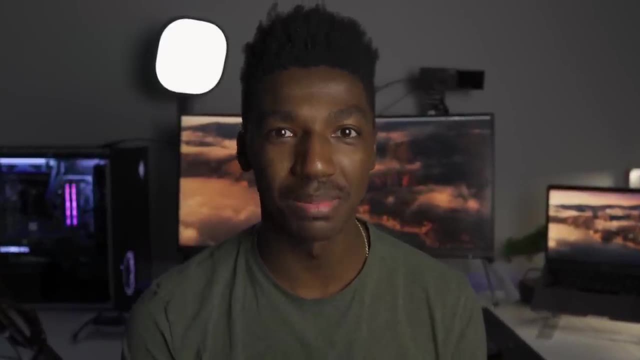 but here are the words. Nonetheless, when you're in this type of environment, you're in a very unique situation to just learn new things. So I mean, if you like learning, that's going to be really fun because you're going to be a lifelong learner is what they call us. So there's that. 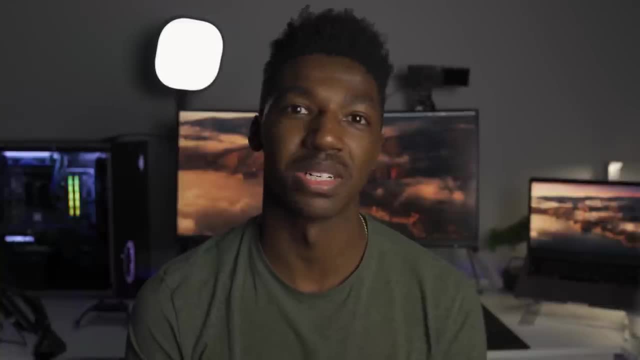 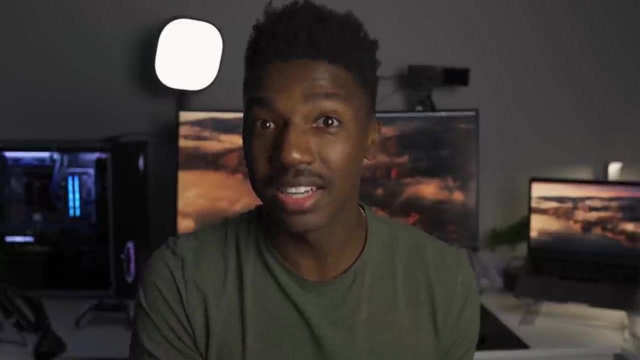 Since starting my career. I picked up JavaScript as my first language And since then I've had to pick up for work Kotlin, MySQL and GraphQL and a bunch of different frameworks like React. I've created a framework like called CodeMandos, but yeah, I've learned and had to learn a ton And I actually 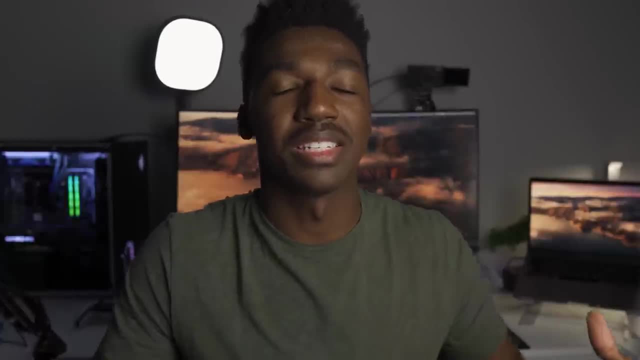 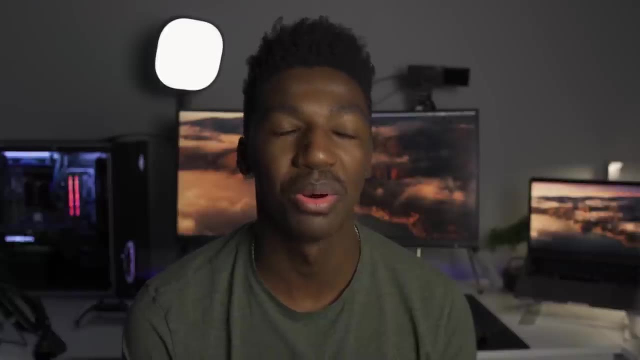 like doing that. before I was a software developer, I used to sit in a chair for twelve and a half hours and stare at screens that just have maps on them And I would go crazy because it was just so boring to me. So I could talk bad about being a software. 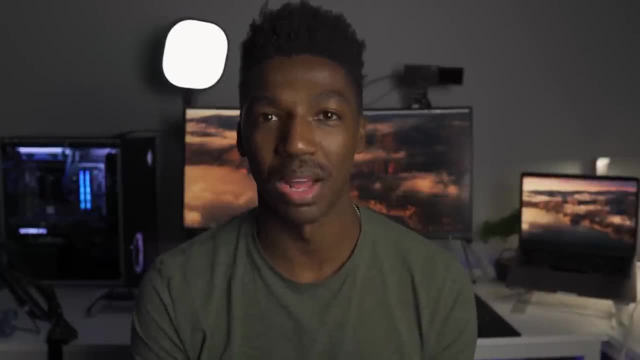 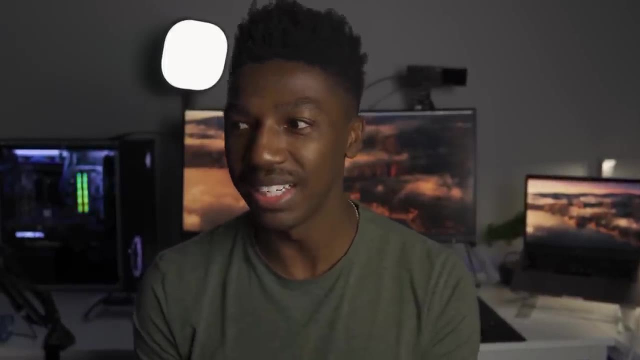 developer all I want, but I could never say that I've been bored at work. I've always had to go to work and solve an interesting and new problem, And it's been that way for the last three years. That's three years of never once having boring work to do. 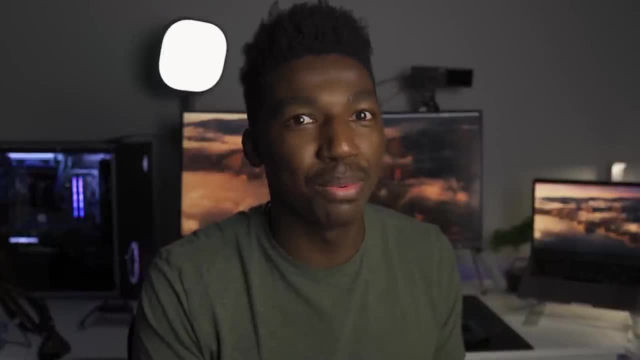 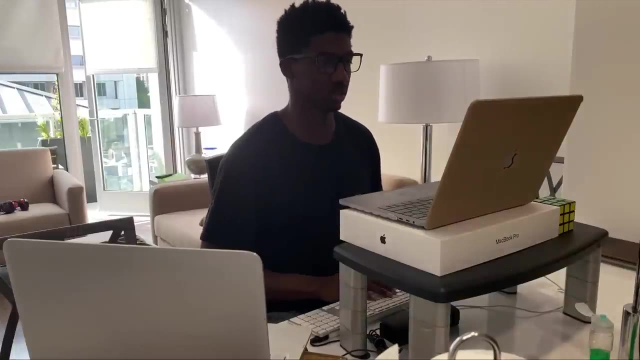 Well, sometimes I have to write really boring tests, but typically 99.9.9, nine point. a lot of the time I'm really having a good time at work and I'm mentally engaged. You know when you're like you're solving a puzzle. 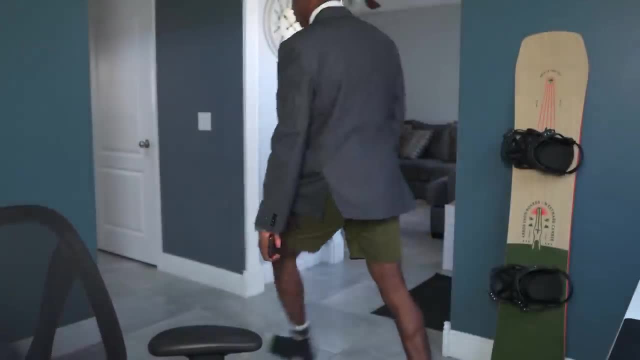 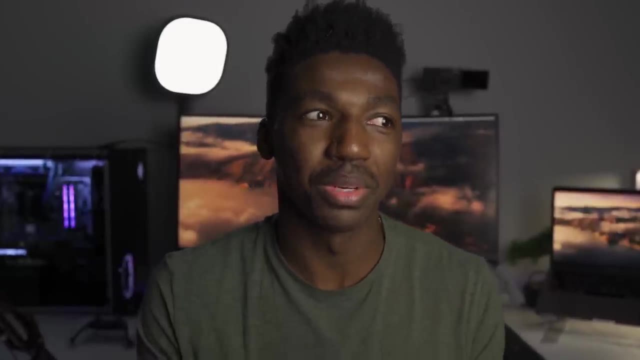 and then you finish that puzzle and you get that boost of like serotonin or whatever chemicals make you happy and excited. you get that as a software developer And that's something that will keep me in this industry, because it's so fun solving problems and creating things. 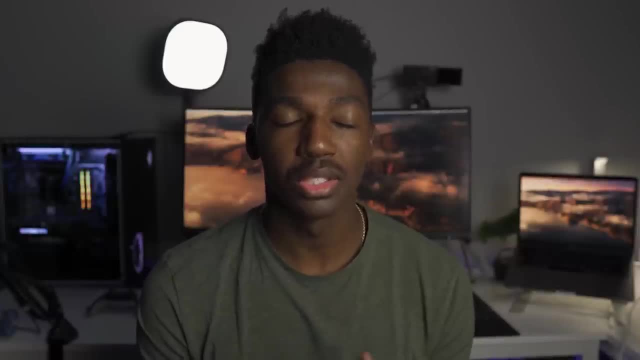 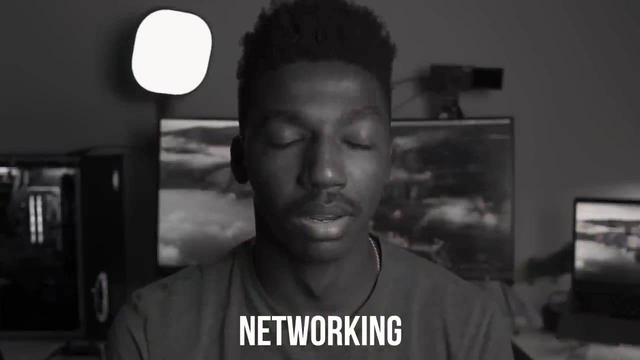 and putting them out into the world. Another thing that I wish I would have known is the super secret cheat code to becoming a software developer, And that is networking And networking. everyone says networking, No, networking Like. there's millions and millions. 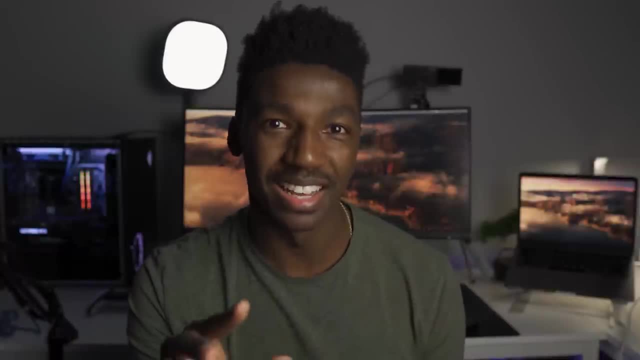 of people, hundreds, thousands, not millions. There's thousands of wannabe developers who are looking to get their first jobs, and there's nothing different about them, But what could be different about them was who they know. I never would have been in the situation I am now. 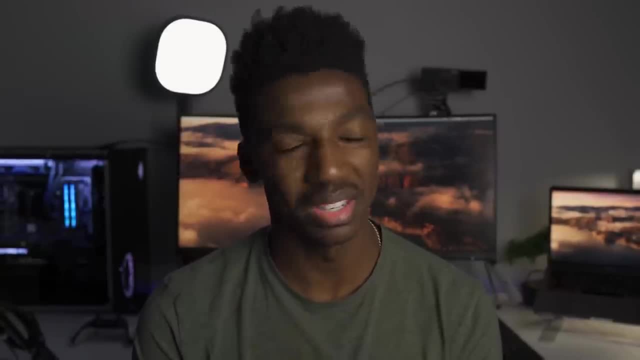 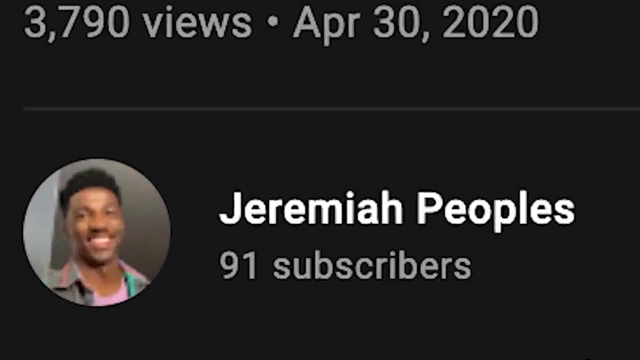 if I had not started this YouTube channel, if I had not gone to Twitter spaces and just started talking in the tech environment. I like to talk about when I was at 98 subscribers way long time ago. Well, like a year ago, A year ago. 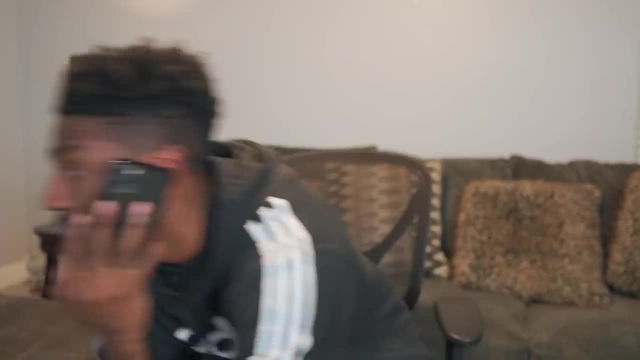 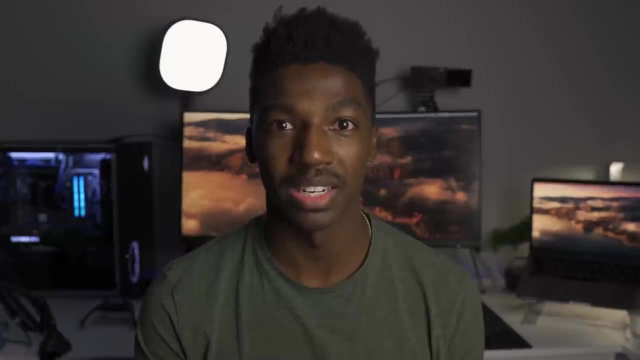 And my dream company from Fang. like the first four letters of Fang reached out to me and they said: hey, we saw your channel. We love that you're a self-taught developer. Would you have a second to talk about setting up an interview? 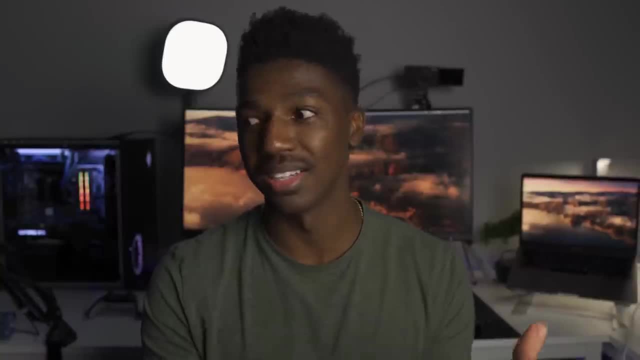 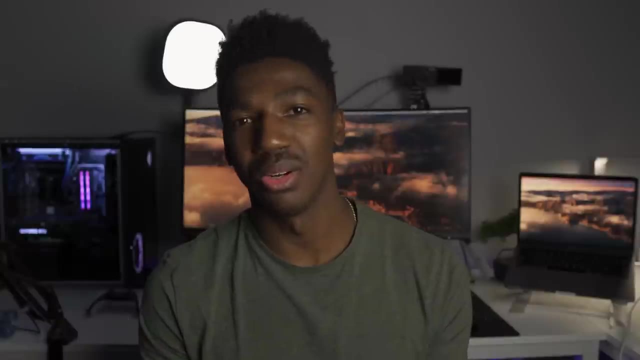 Which is wild to me, And that was only possible because of the networking thing that I didn't know. YouTube was technically a networking thing And not everyone needs to start their own YouTube channel or have their own blog. I don't like when people say that. 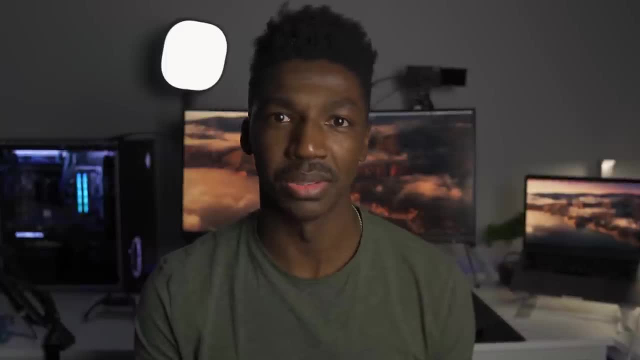 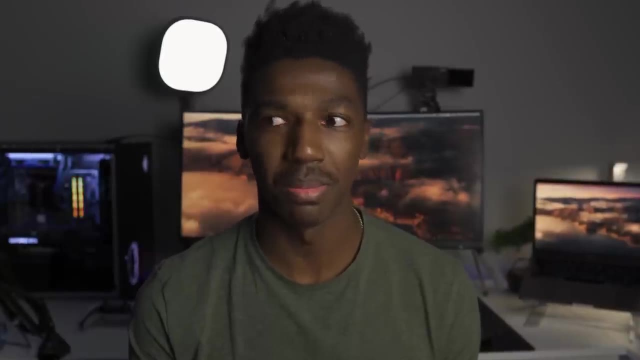 But try to take advantage of things that that interest you. So if you like making mobile applications, go to a mobile application meetup. If you're looking to build a project and you need some help, ask some people for help. There's a ton of developers who want to get connected. 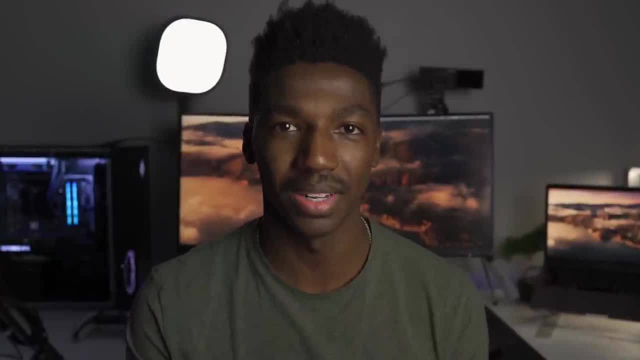 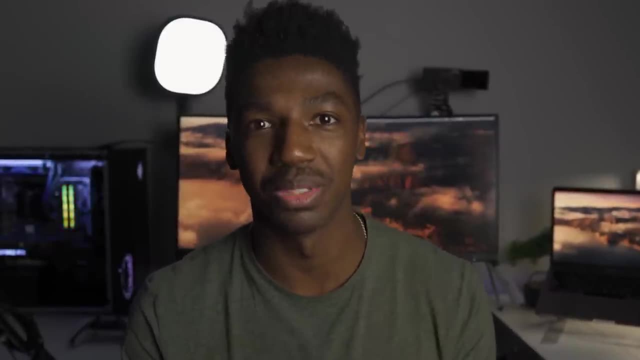 in this community. So moral of that story is: don't just network to network, Rather network because there's something interesting to you out there that needs other people, or you want other people to check out, because it's cool or they can help you out somehow. 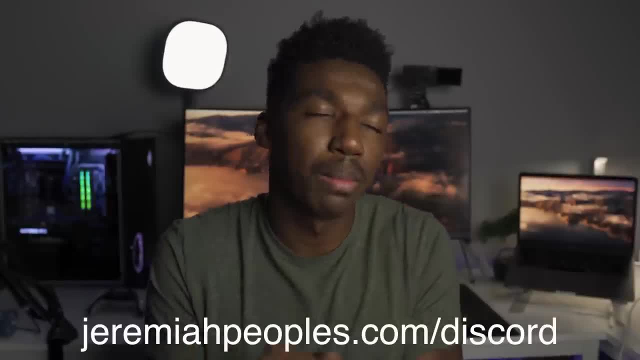 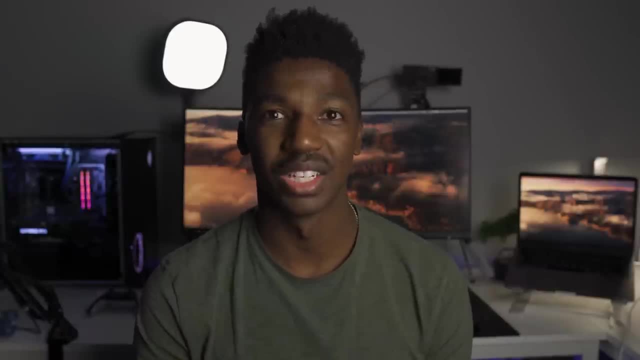 And speaking of networking, I do have my own little developer discord channel where we chat about code stuff and tech stuff and tech news and articles like that, So you're welcome to join that in the description as well. And the last thing that I wish I would have known: 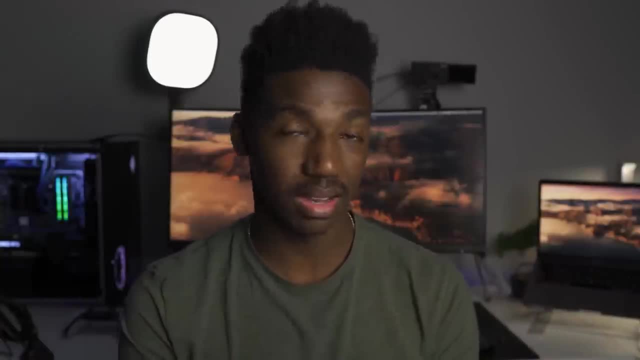 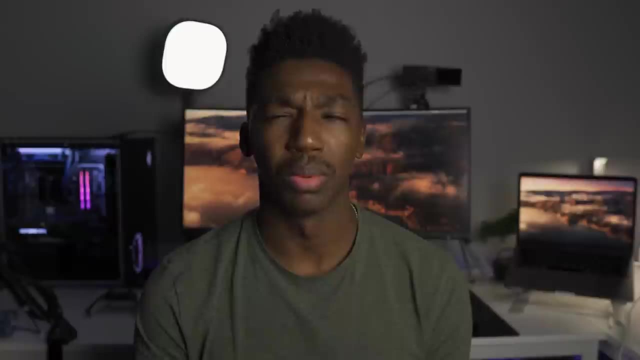 that made my little top five video is that being a software developer or learning how to be a software developer is not the only means to get into the tech industry, Which is super weird to me, because whenever I think of tech or the tech industry and the people in the tech industry, 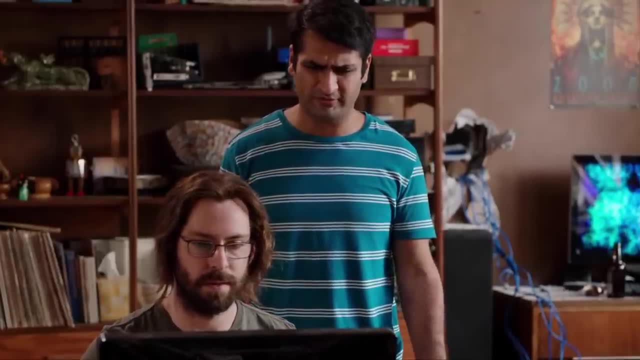 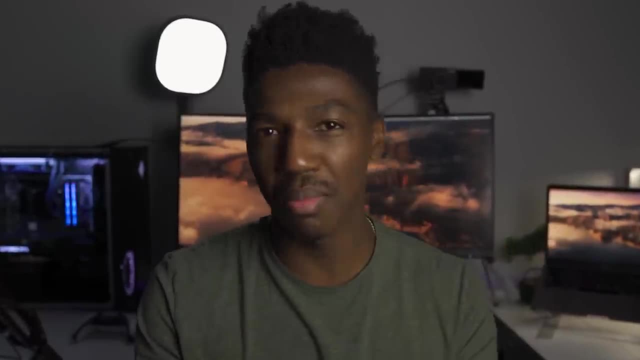 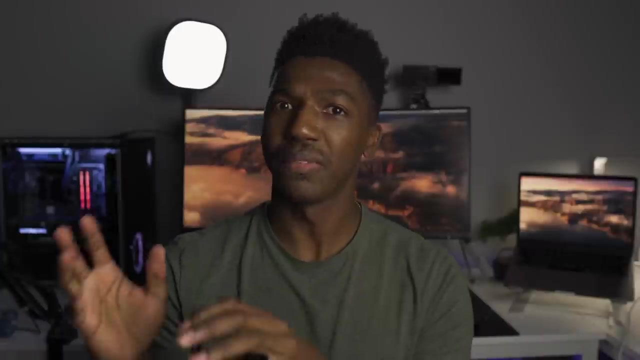 I think of software engineers, software developers, people who can code tech, But apparently there's a good handful of other careers that are almost like software developers. They're almost techie and they are really important to creating a whole technical product. So if you tried out coding because that's how you wanted, 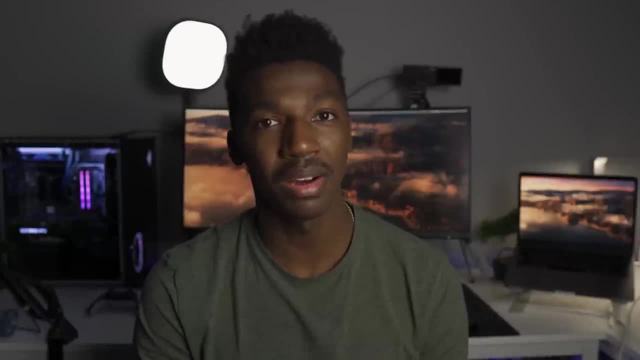 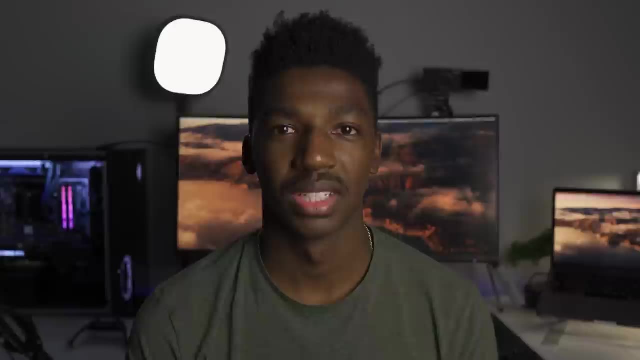 to get into tech and that didn't quite work out with you because you didn't like coding. you're not out of luck. There's a lot of other different career paths that can still point you into creating technology. So the most common career fields that are in tech: 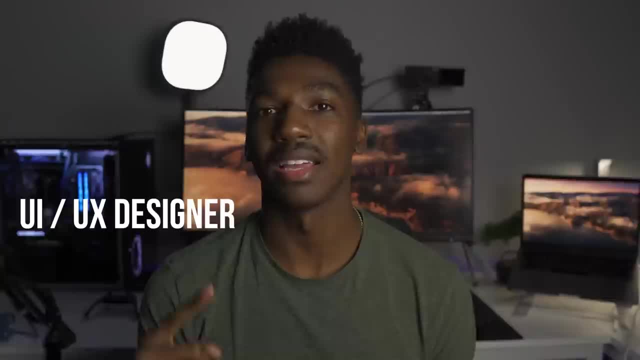 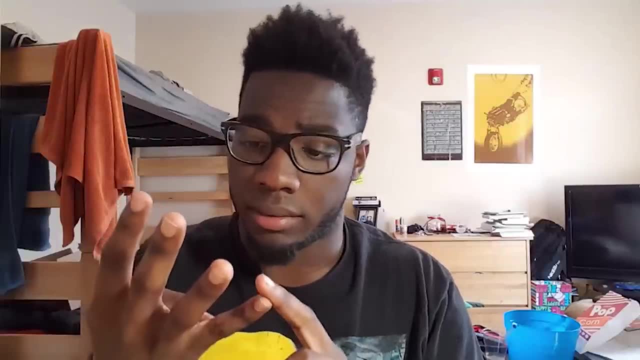 but not coding- are UI UX designer and product manager. UI UX design is actually a really cool pathway to get started in tech. I actually have a fourth brother who's just starting his career in UI UX And essentially you're just all swagged out. 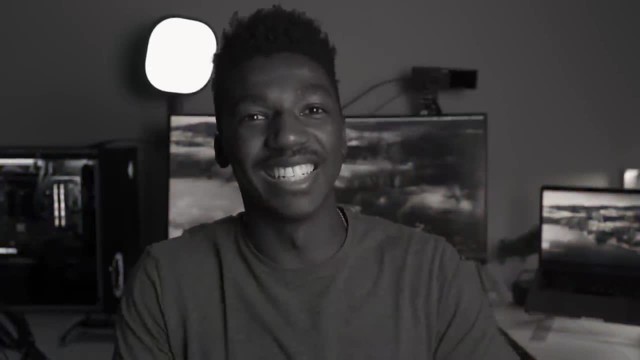 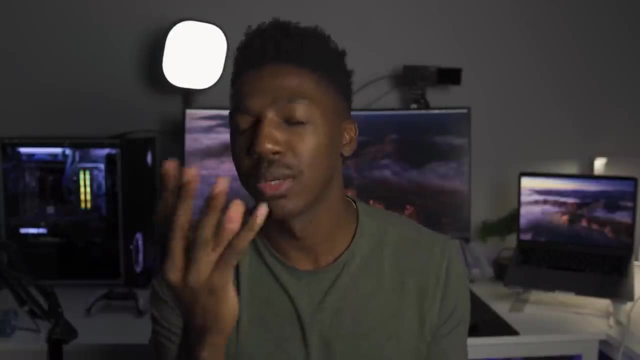 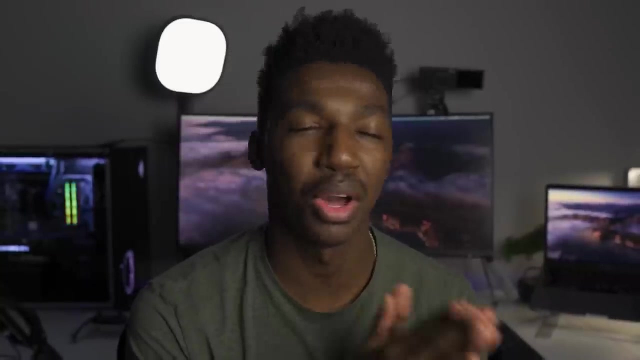 when you come into work with your Gucci belt on UI. UX designers are incredibly important when it comes to creating a beautiful application that people actually like to use. So me as a software engineer- I could write the most beautiful code. It works so efficiently. 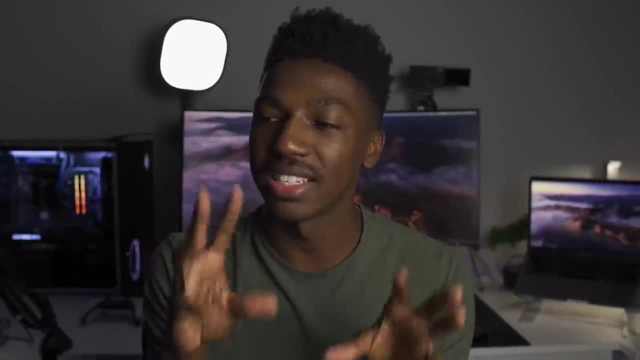 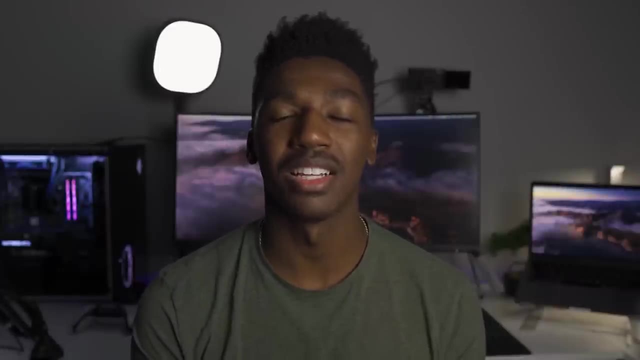 but if it looks like I made the application with two center blocks for hands and I have no design at all in it, no one's gonna use my application. That's why UI UX designers come in clutch, because they really understand the users. They understand what the users want. 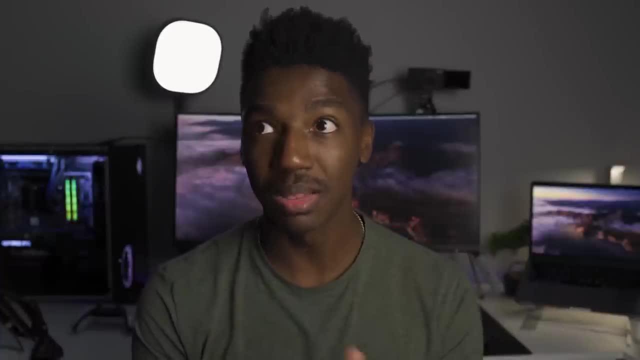 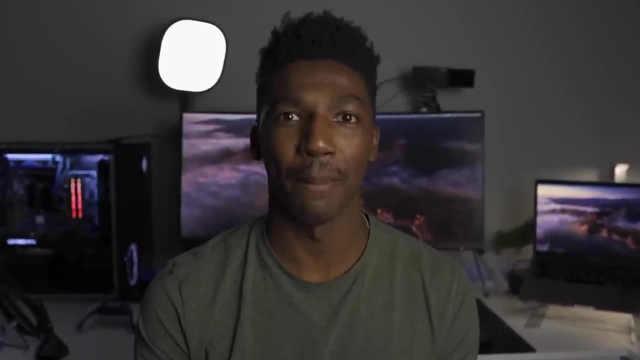 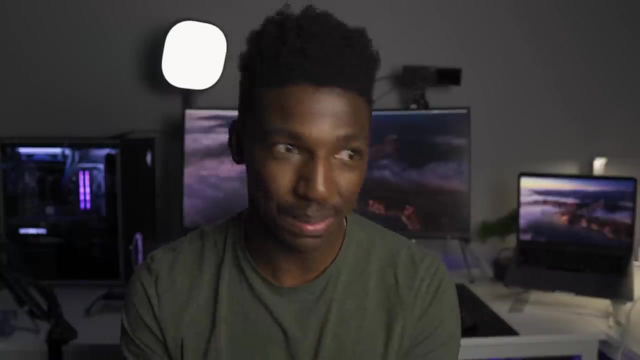 and they can display that and communicate to that, to the development team And to the product managers. And speaking of product managers, product managers are people who like managing, but the project that they're typically managing is a technical project. A technical project has a ton of spinning wheels. 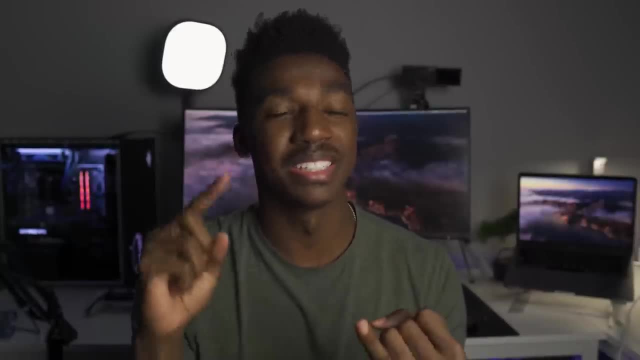 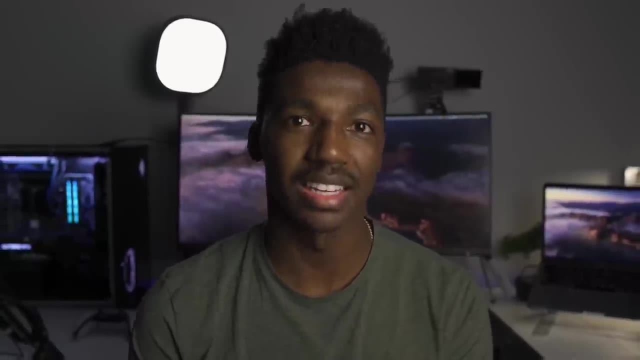 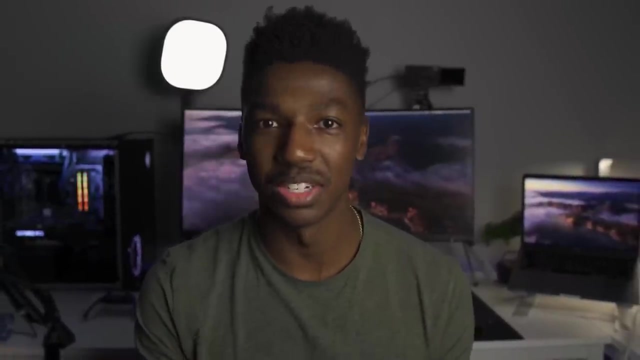 that they need to manage. The biggest spinning wheels are managing the software developers and managing the designers, So product manager type people are incredibly important to make sure that you're hitting deadlines, The tasks are getting completed in the correct order and that the application is meeting the needs of the stakeholders. 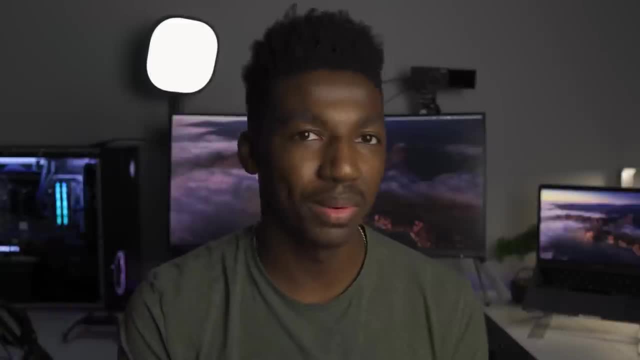 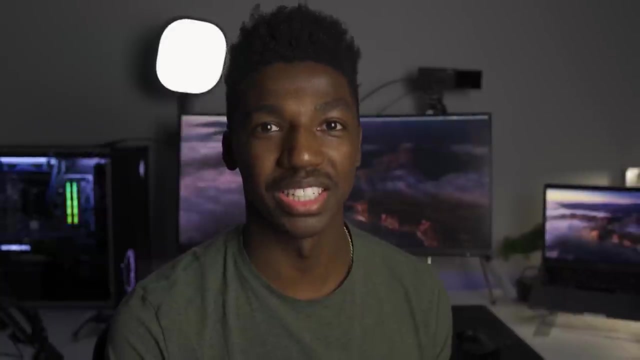 and the people who are actually funding this project. So, whether it be software development, UI, UX designer or product manager, all of these career fields are super important in creating nice applications. So those are all the things that I wish I would have known before starting my career becoming a software engineer. 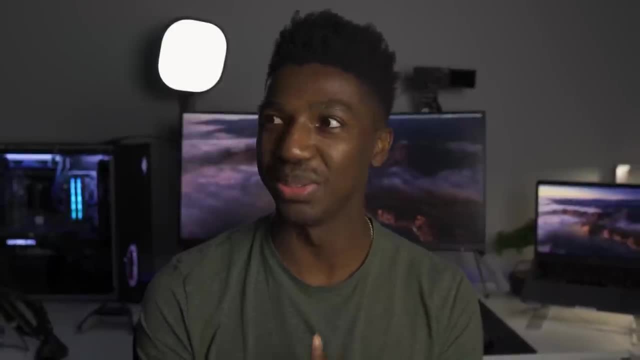 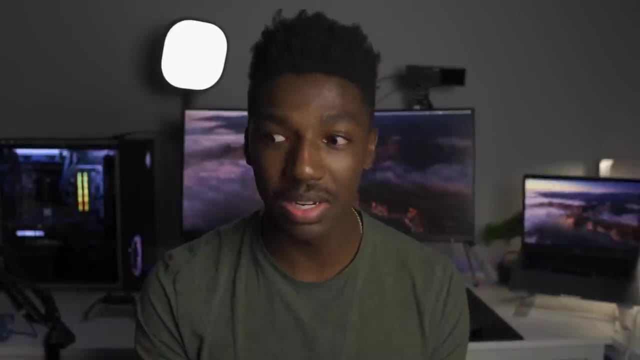 I'm really glad that you watched the video. I hopefully you gained a lot of value from all of the things that I picked up over these three years. Thank you so much for watching. I will see you on the next one, And I think that's all the words I have to say. See you.